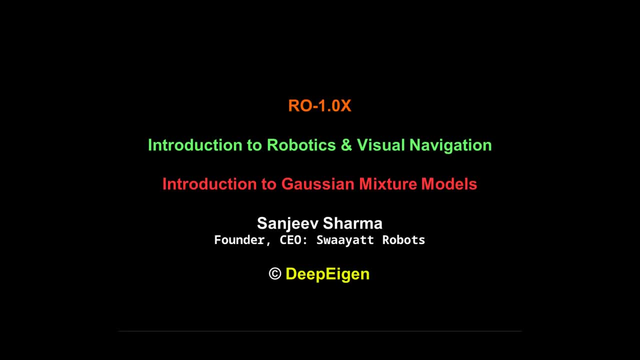 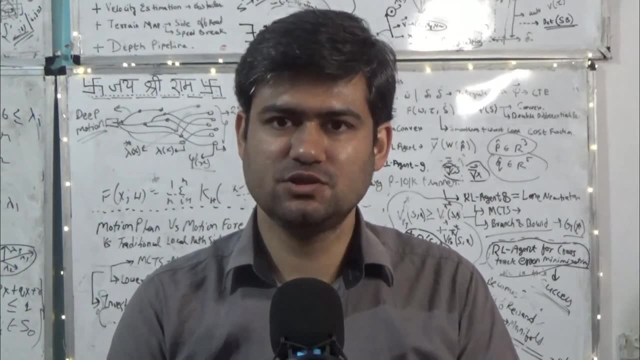 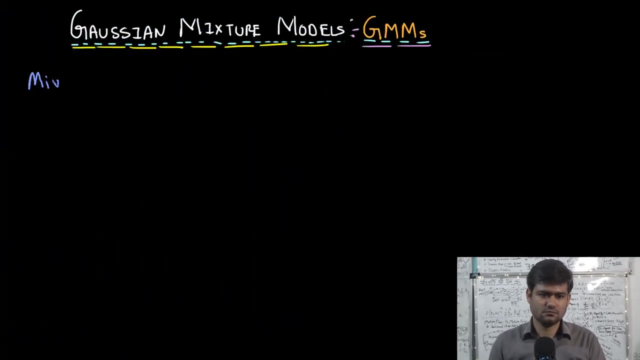 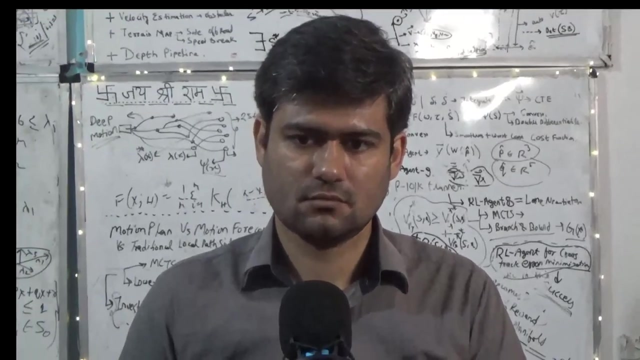 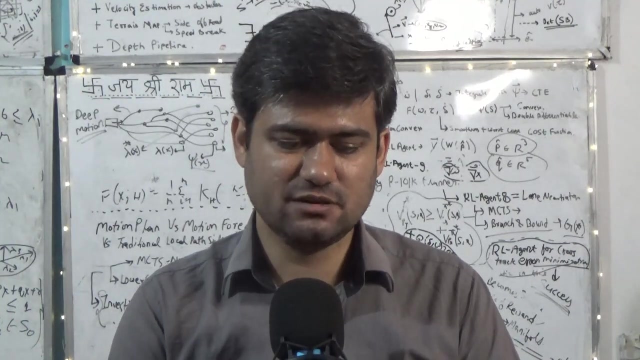 Hello everyone. In this lecture we are going to discuss another clustering algorithm known as the Gaussian mixture model or GMM. So Gaussian mixture model is an instance of much broader topic known as mixture models in the machine learning literature. So in this lecture we are going to discuss GMM, which is an instance of much broader topic known as mixture models in the machine learning literature. 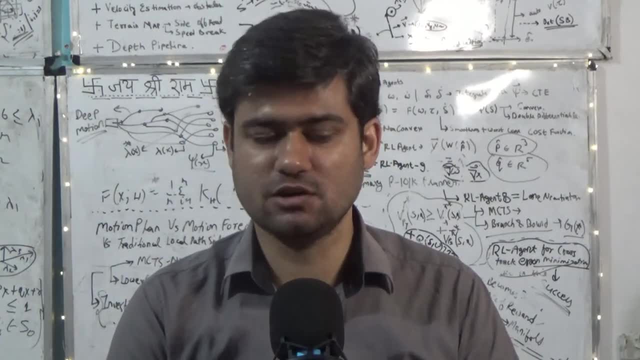 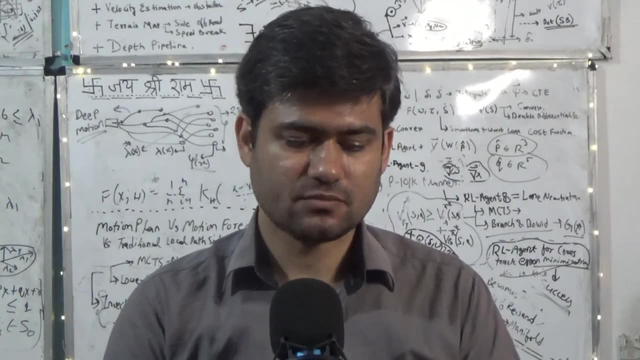 where in GMM the underlying data distribution is modeled or approximated as a simple linear superposition of the Gaussian components of the GMM. So it can be used to model or approximate. It can also be used to estimate the multimodal distributions that generated a data set. 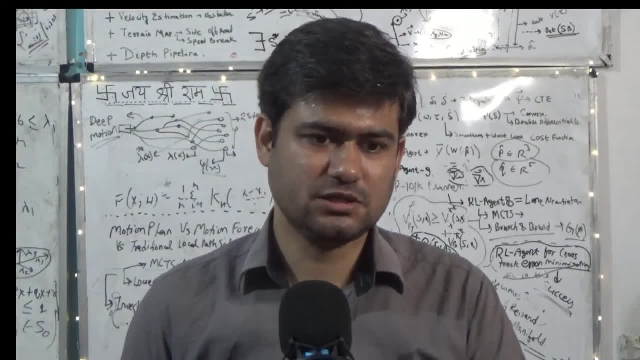 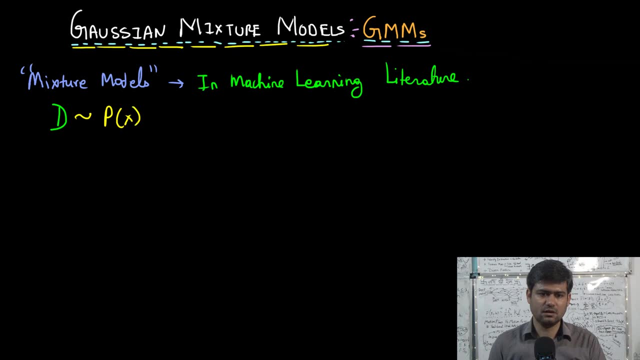 So let's suppose if we have a data. So let's assume that we have a data set and this data set is generated from some distribution P of X, where the data set contains M data points, X, I, Where each of the X- I is an n-dimensional real vector. 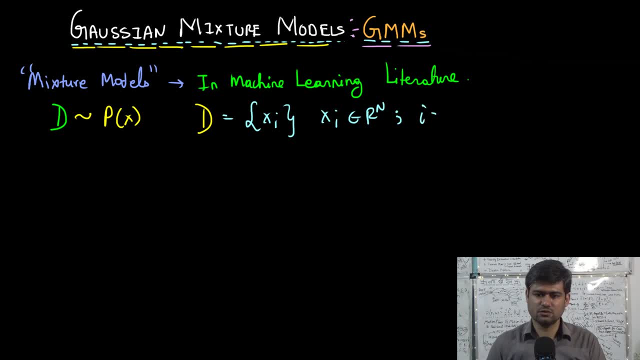 And the And I goes from 1 to M. That is, in this data set D we have M data points where each of the data points is an n-dimensional real vector, And this data set is sampled from a distribution P of X. 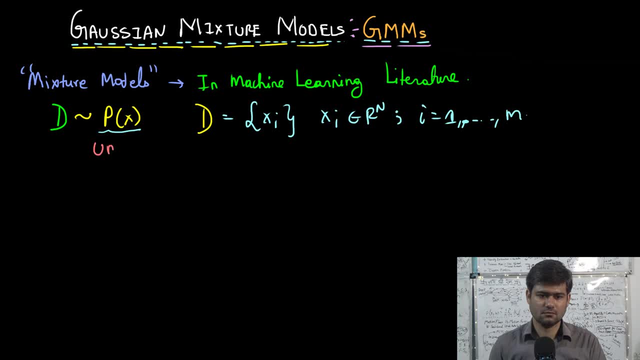 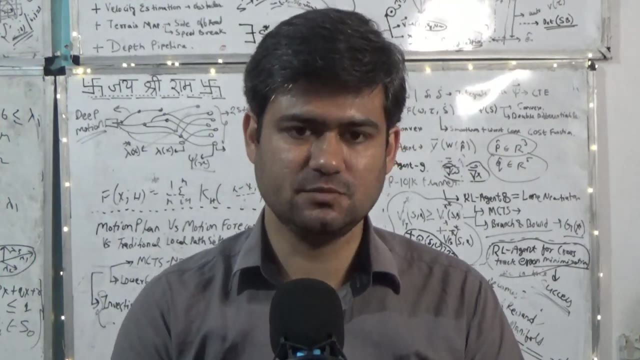 So there's an underlying true distribution. So P of X is the underlying true distribution which you do not have access to. But what we have access to is a data Sampled from that distribution or generated from the distribution So we can use the Gaussian mixture model to model or approximate. 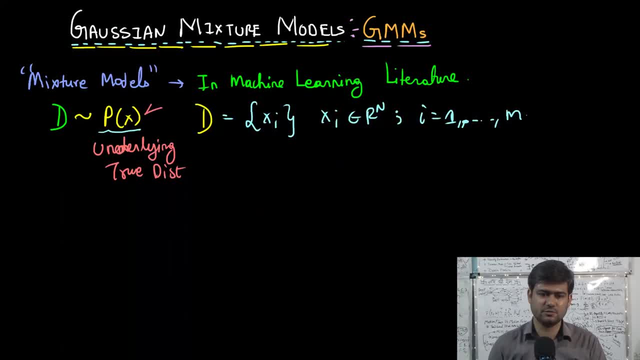 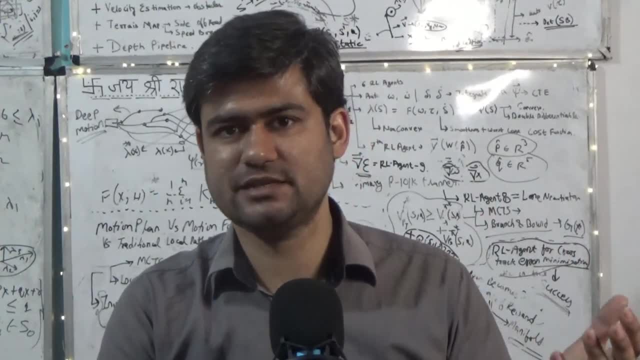 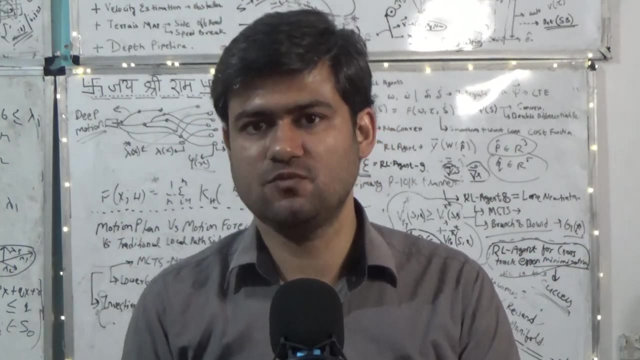 The underlying complicated or perhaps a multimodal distribution that generated the true data set, Just like what we did in the kernel density estimation. So in kernel density estimation we have data set which is generated by some multimodal density function- P of X- But we didn't have access to the true density function. 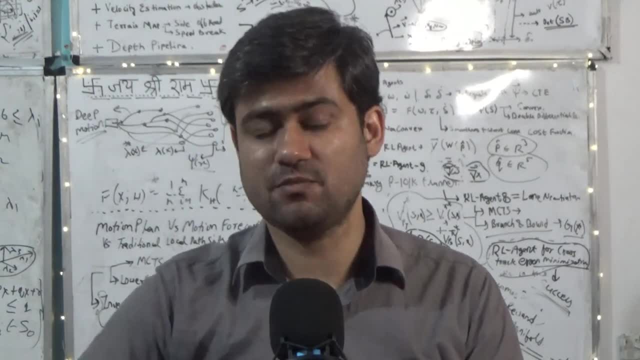 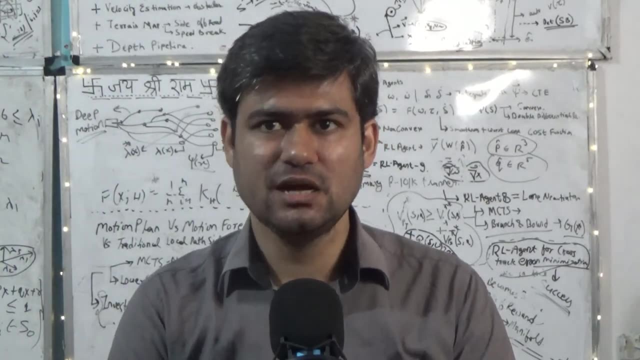 What we have, what we had access to, was a data set sample from that density function Or that distribution. So we estimated that distribution using the kernel density estimator function and then we found the modes of the kernel density estimator function and then we use those modes to cluster data set. 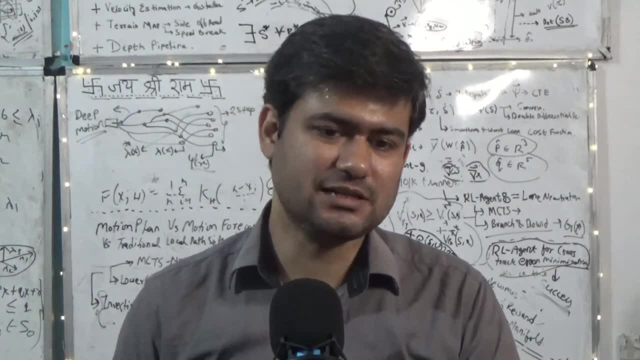 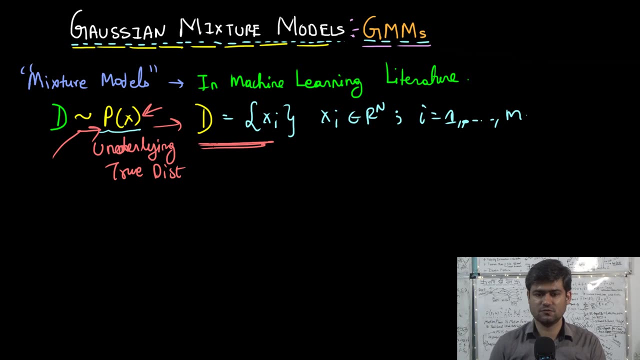 So similarly, we can do the same thing in the GMM. So we have access to the data set, but we do not know the true density function or the distribution function that generated this data set. But since we have access to the data set, we can use this data to approximate this underlying true density function or this distribution. 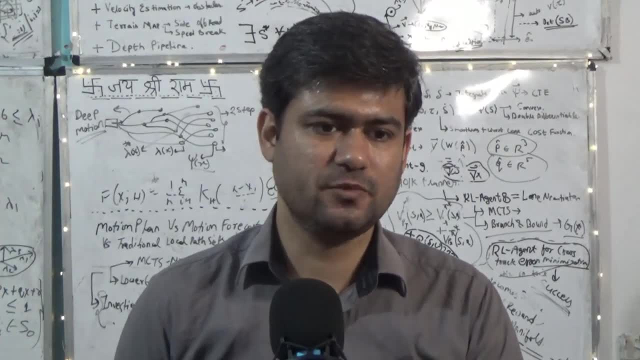 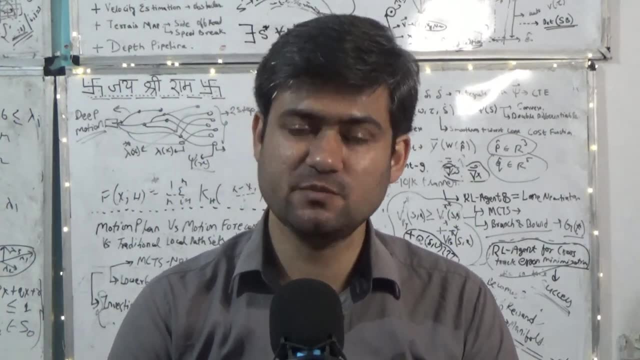 So GMM is an instance of unsupervised machine learning algorithm. So all the previous clustering algorithms- the k-means clustering algorithm and the kernel density estimation based mean shift algorithm that we have learned are an instance of unsupervised machine learning algorithms. 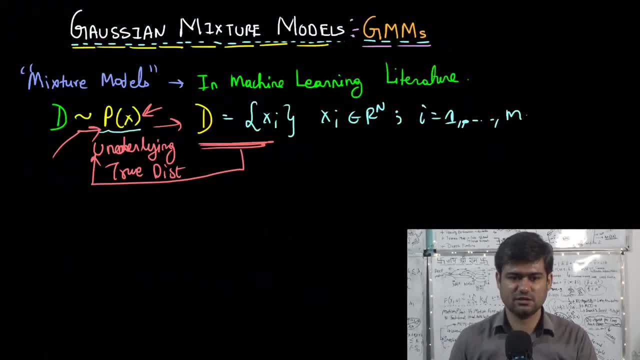 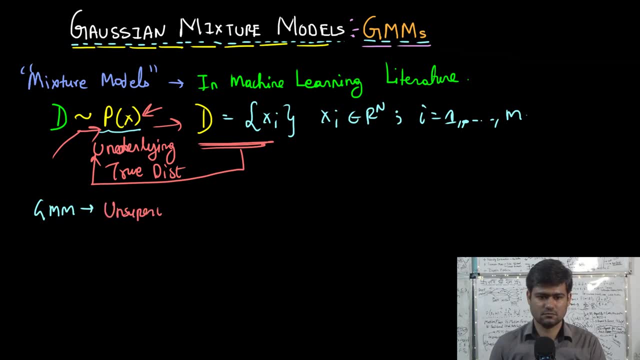 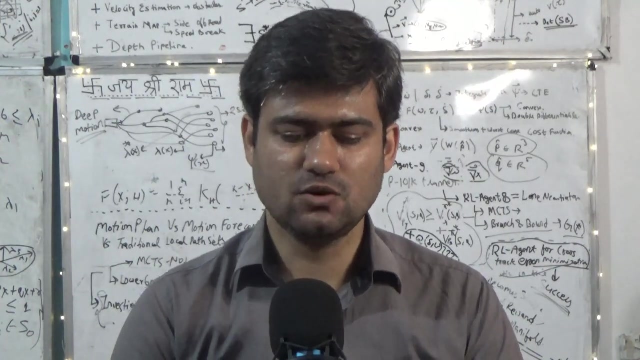 Similarly, the Gaussian vector model here is also an unsupervised machine learning algorithm, So we can use this data set. So it is an unsupervised machine learning algorithm where, similar to k-means clustering or the kernel density estimation based clustering, the goal here is to identify the number of components or clusters in a given data set. 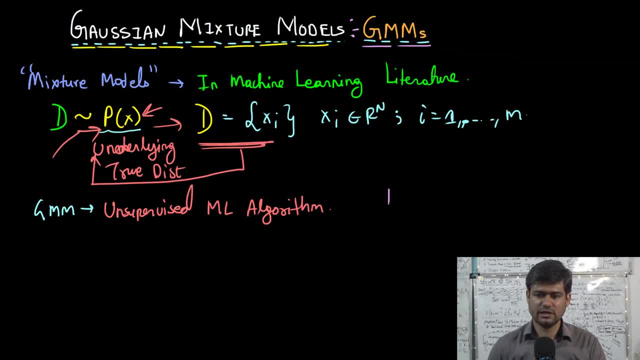